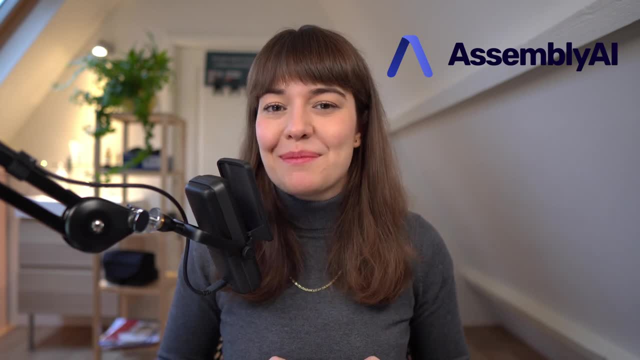 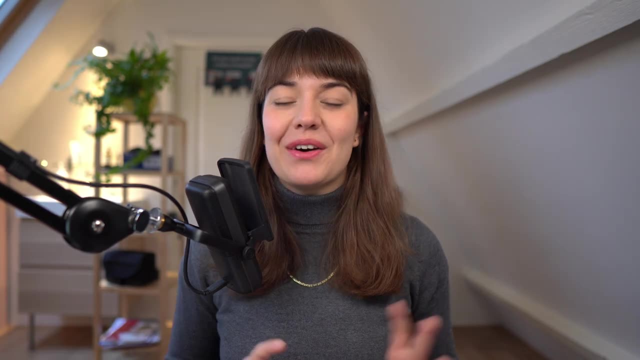 Assembly AI is a company that is making a state-of-the-art speech-to-text API. If you want to try Assembly AI yourself, you can go grab a free API token using the link in the description. All right, let's start with bias. So bias is basically the amount of prejudices. 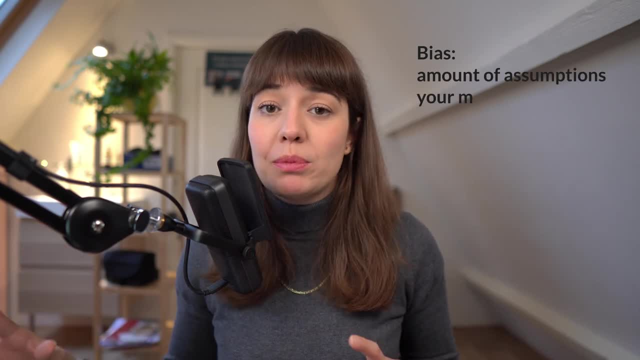 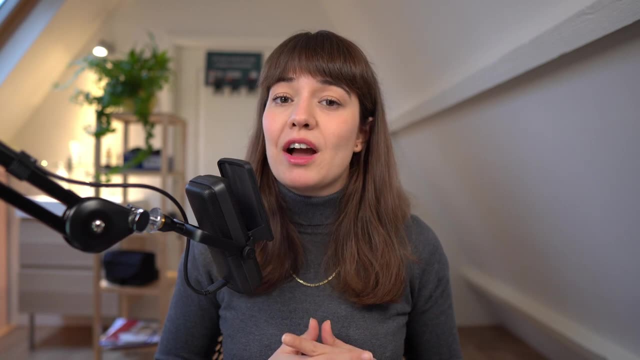 or assumptions your model is making against a certain problem that you're trying to frame. The more assumptions your model has, the higher the bias is going to be on your model. One model with a very high bias is linear regression. The reason linear regression? 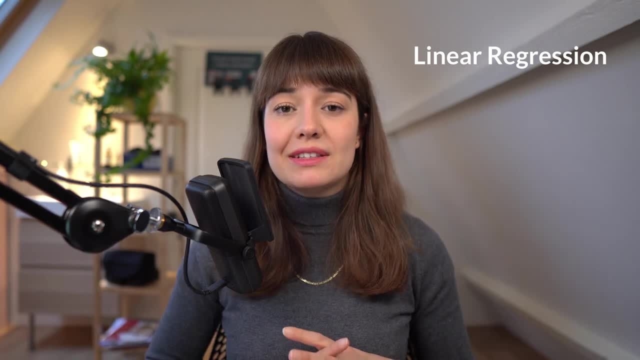 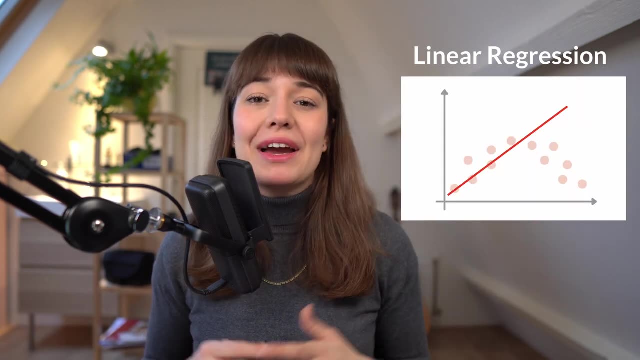 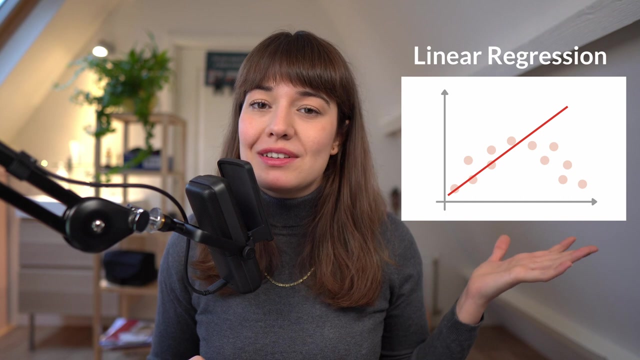 has high bias is because it assumes that the data has a linear distribution. And what happens when you give it data that is not linear is this: You might not be able to fit the data at the end because of all the assumptions that you're making about the problem or the data. And what does this? 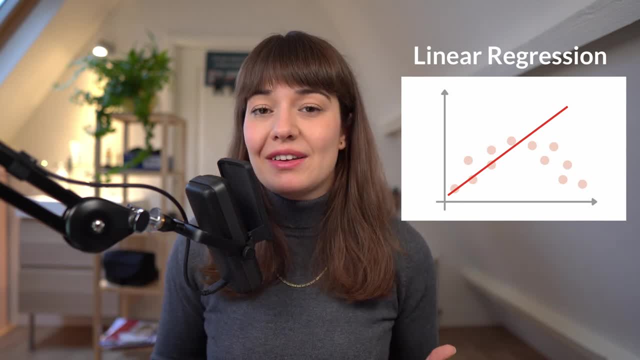 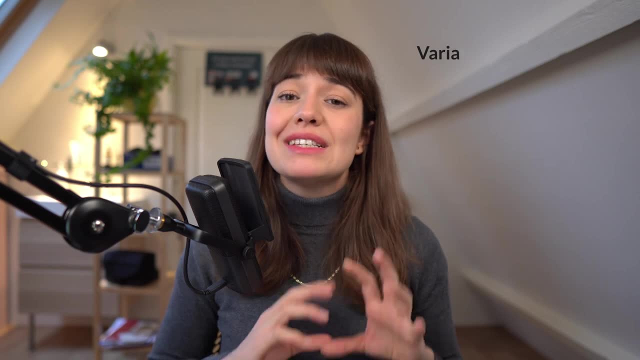 look like You might have seen before. It looks like underfitting. So that's why high bias- so a lot of assumptions- means underfitting. Variance, on the other hand, shows us the sensitivity of your model on the training data, So it tells us how much the output would have. 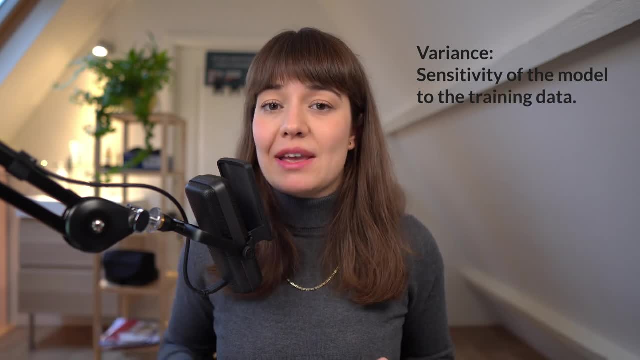 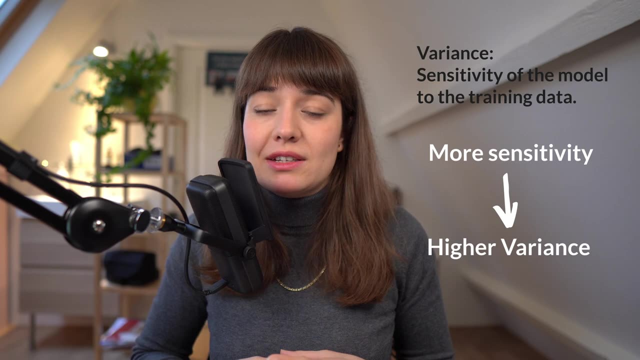 changed if we change the training data. even in the same problem, When the model is dependent on the subset of the real world that you're training it on, what happens is if you change that subset in the real world that you're selecting to train it, the outcome is going. 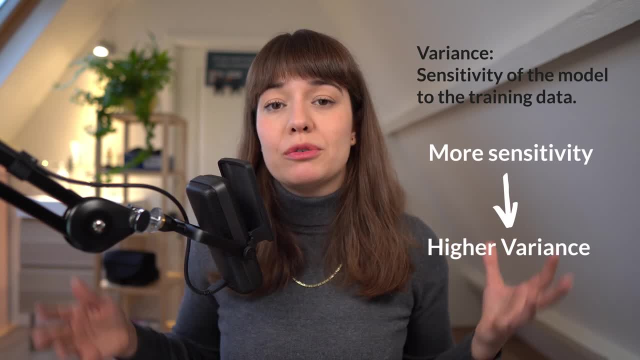 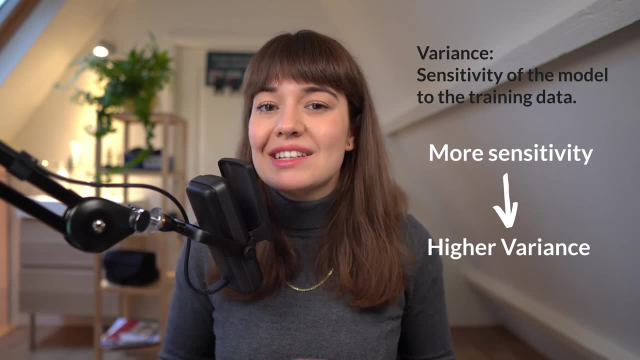 to change dramatically. A model like this will not be able to perform well in the real world. So what you have at the end is a model that is overfit to the training data. So, as you can imagine, high variance means overfitting. Models that have high flexibility tend to have high 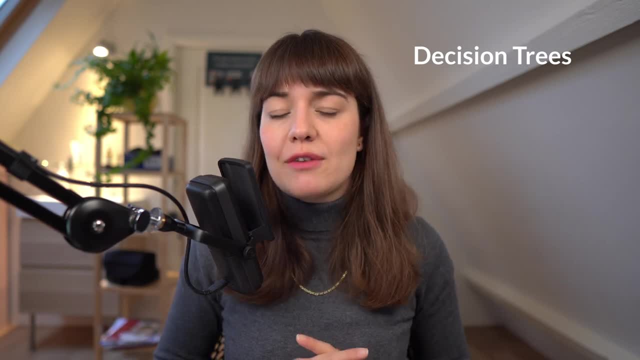 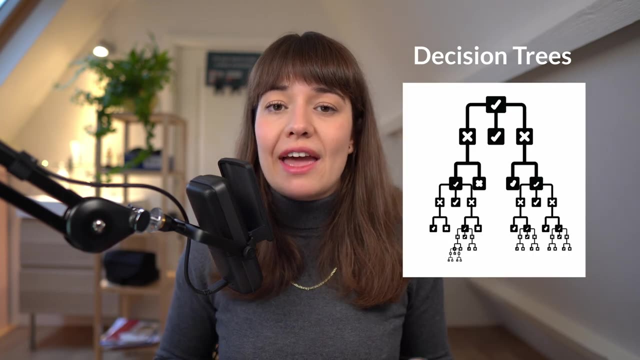 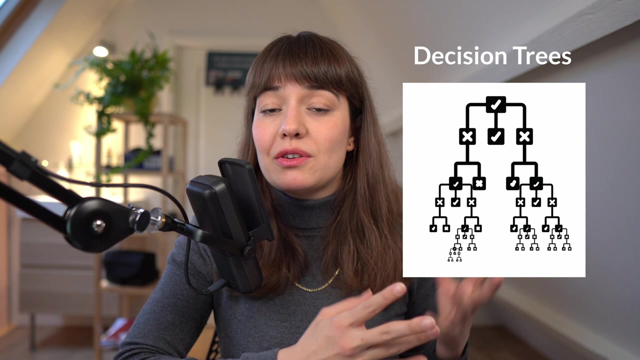 variance, like decision trees. So if you imagine a decision tree, if you do not put any limitations on this tree, it will grow and branch up as far as possible to fit all and every single data point as possible. While training a model like this that has fit every single data point, would give us 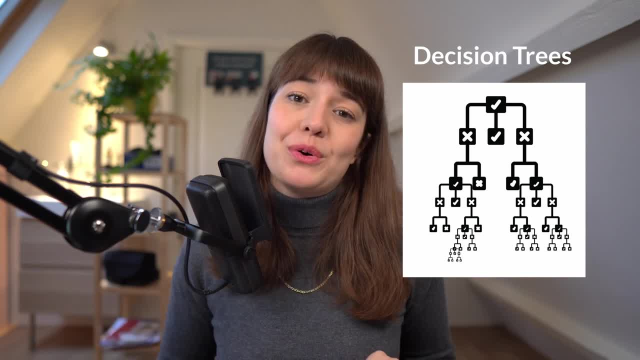 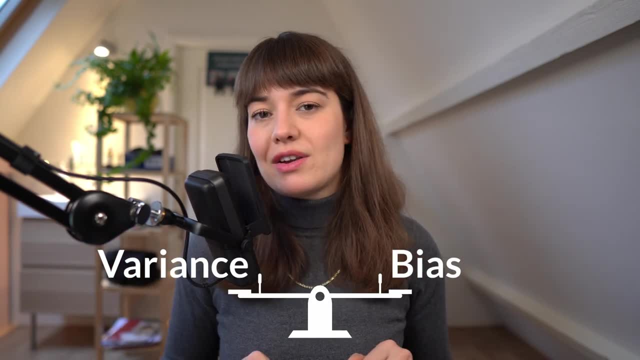 really good results, but in the real world it will fail to perform. With traditional machine learning algorithms there is always a little bit of a problem. So what you have to do is a little war between lowering bias versus lowering variance, because when you try to lower one, 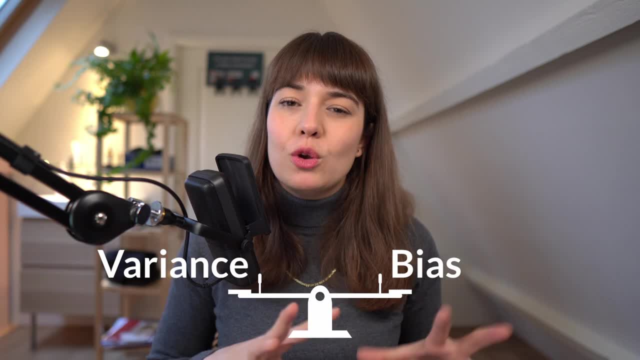 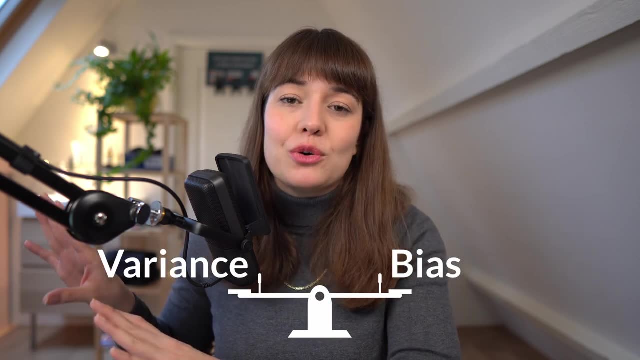 the other might shoot up, and you want to strike a balance there. You're always trying to fit the data well enough so that you're not underfitting, but at the same time not overfit the training data, so your performance in the real world is still protected. This is called the bias, and 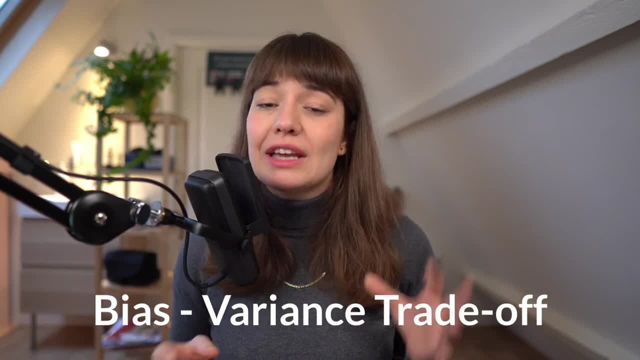 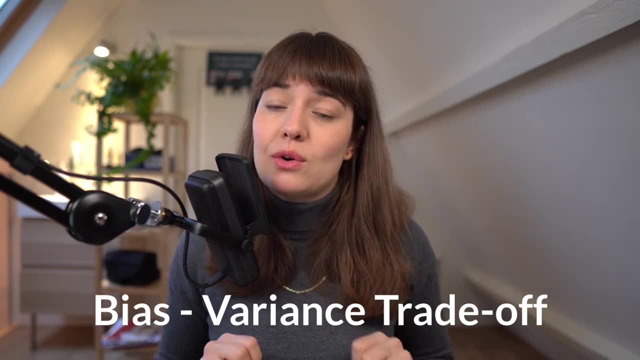 variance trade-off. But with the latest development in machine learning, especially with deep learning, we don't really have to worry about that anymore, because we have some tools in our hands that will lower bias only or lower variance only. So let's talk about some of those solutions. 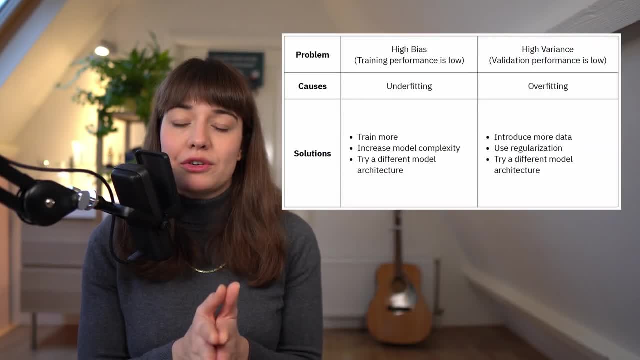 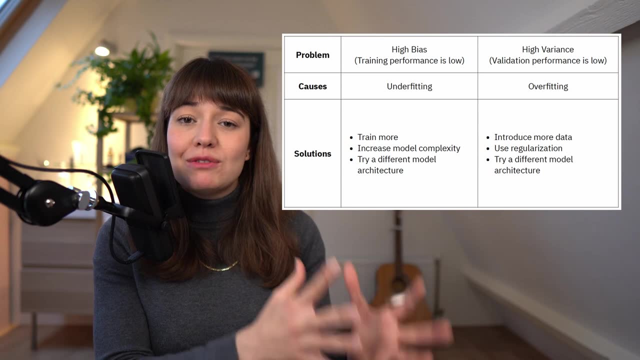 If you have high bias, as we said, what that means is that you're underfitting, And one of the best things and first things you can try is to train your model more, because maybe you have just not trained your model enough and your model did not have yet time to converge to a good solution. 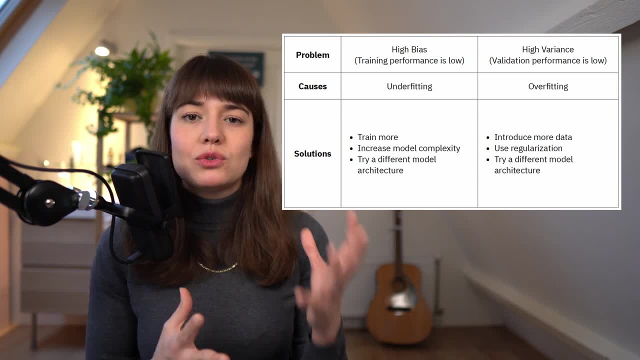 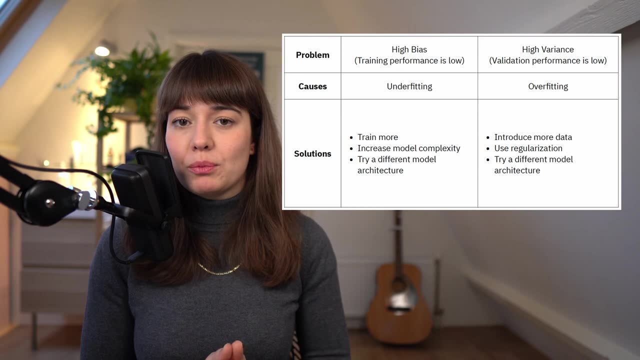 And that's why you're underfitting your problem. So trying to train it a little bit longer might help you solve underfitting. Another thing you can do is to try increasing the complexity of your model, because maybe your model has way too many assumptions and is way too simple for the data that you're trying to frame. 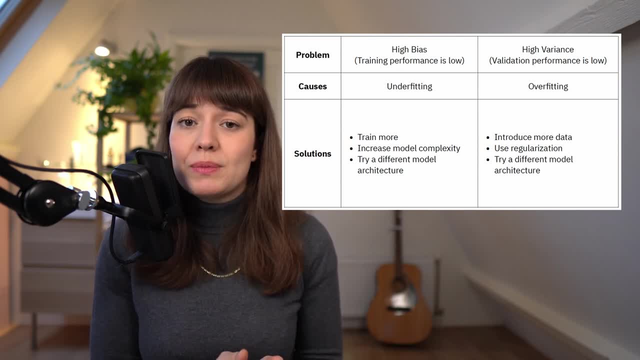 So this might look like: if you have a decision tree with maximum depth set to two, increasing that to five or ten, That will create, that will make your model a bit more complex and at the end, it will lower your bias. Another thing you can do is to change the model architecture that you're using. 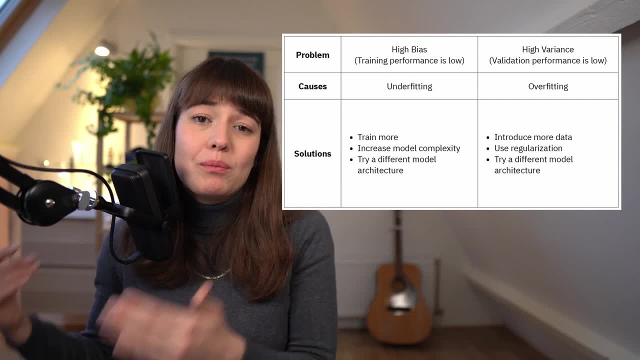 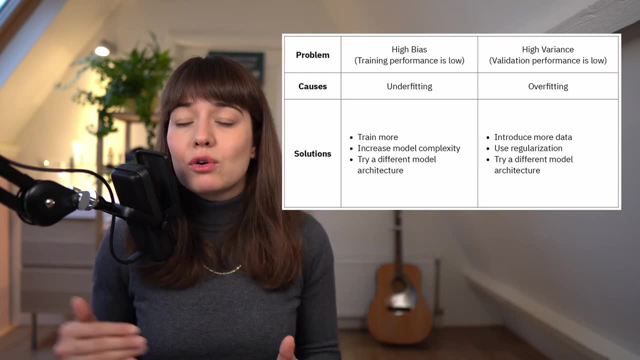 Maybe you are using a architecture that does not fit your model. So, for example, maybe you're doing image classification with deep neural networks, but maybe trying a convolutional neural network architecture would work better for you and you might not underfit at the end. 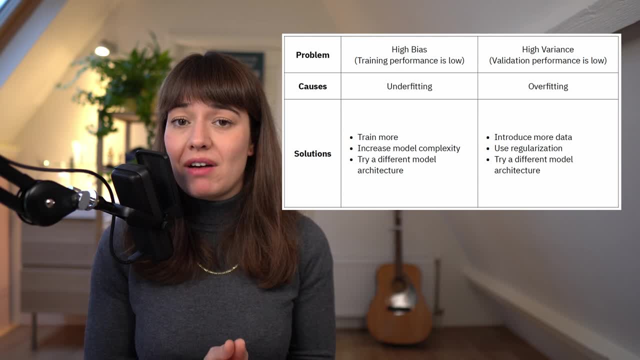 Next, we have high variance. And what kind of model do we have when we have high variance? It is a model that has overfit. One of the first things you can do is to try to train it with more data if you can't. This might not be possible always, because sometimes getting more data is basically too costly or not even possible. But if you're overfitting, introducing more data to your training, if possible, is always a good idea. Another thing you can do is to use regularization on your model. 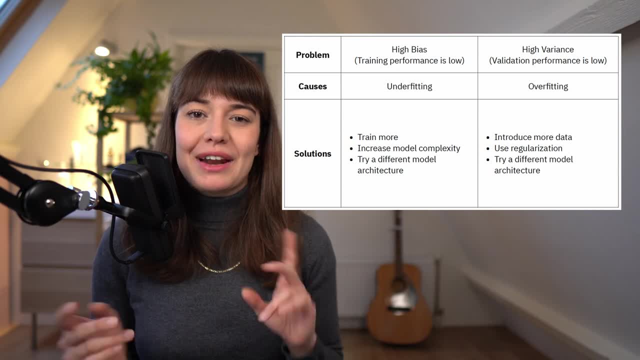 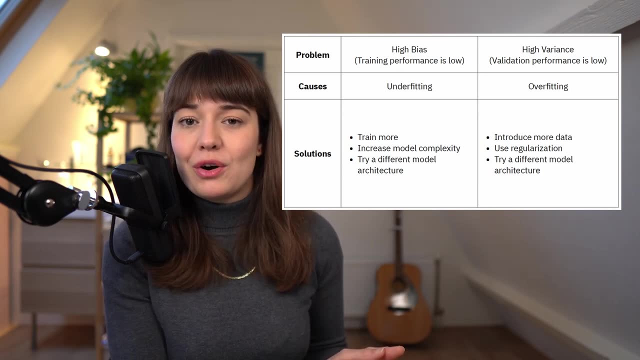 So what is regularization? We talked about this in a previous video and I will leave the link to it somewhere here. But basically, regularization, what it does is lower the complexity of your model. So you can see, it's basically doing the opposite of what we did when we were trying to deal with high bias. 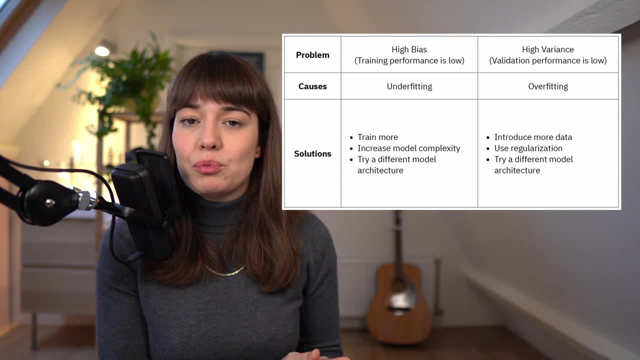 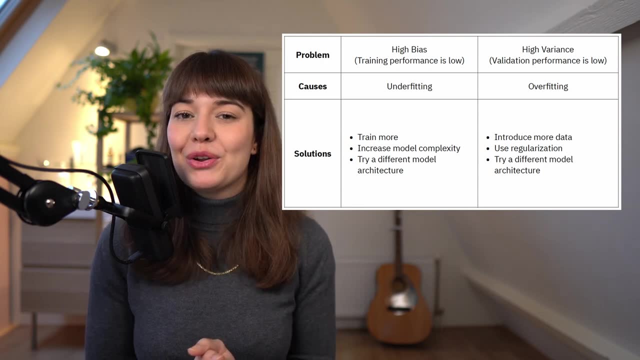 By using regularization, you will be limiting the flexibility of your model or the complexity of your model, of your model, basically decreasing the complexity of your model and will be able to lower the variance in your model. And lastly, again, you can try a different model architecture, Maybe the model 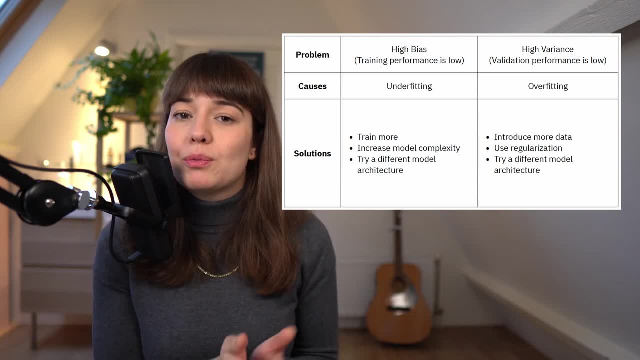 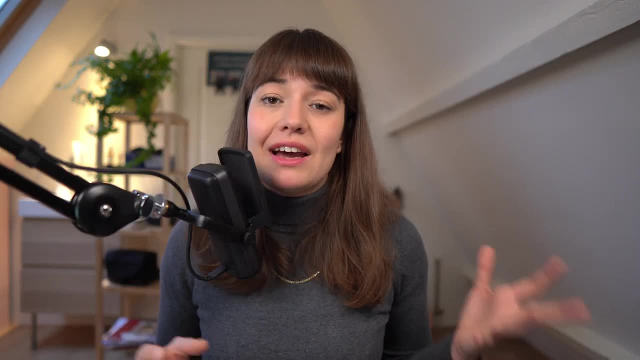 that you're trying to use right now is just not a good fit for the problem that you're trying to frame. So trying out a different model architecture might help you combat overfitting. As I mentioned now, there are ways to lower bias without increasing variance, and vice versa, So one way to do that is. 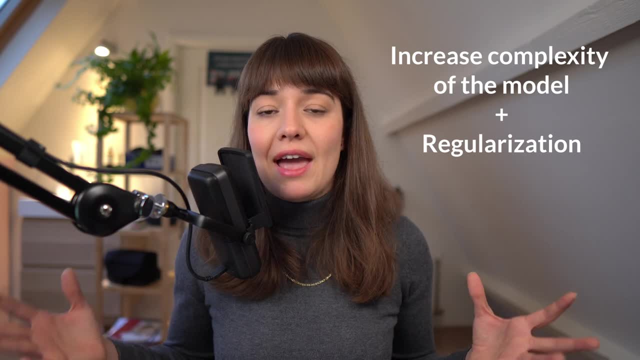 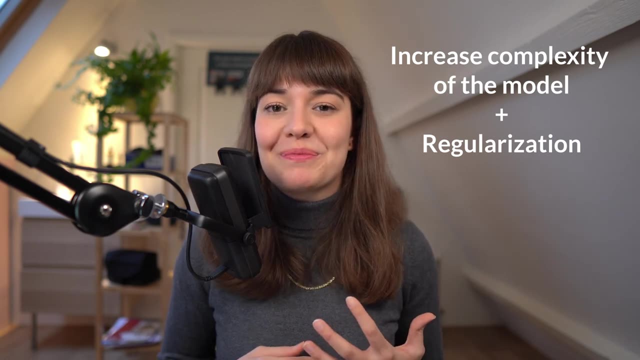 if you're underfitting, you can increase the complexity of your model and use regularization on top to avoid overfitting. that comes from the high variance of increasing the complexity of your model If you're overfitting. on the other hand, if you introduce more data to your training, 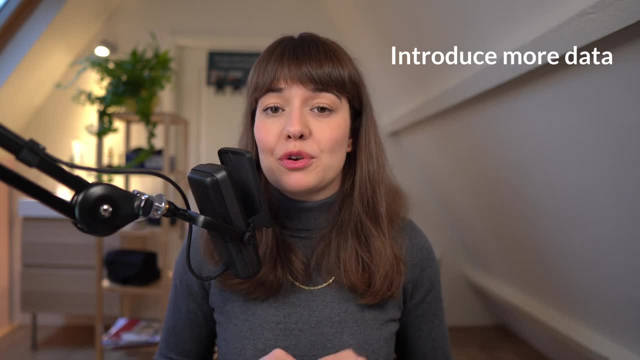 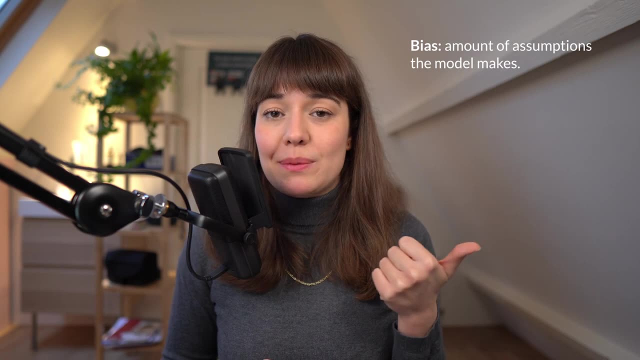 you will be lowering the variance without increasing the bias of your model, And that's it. That's all you need to know about bias and variance. Let's do a quick summary. Bias is the number of assumptions that your model has. If it has too many assumptions, it will have high bias and 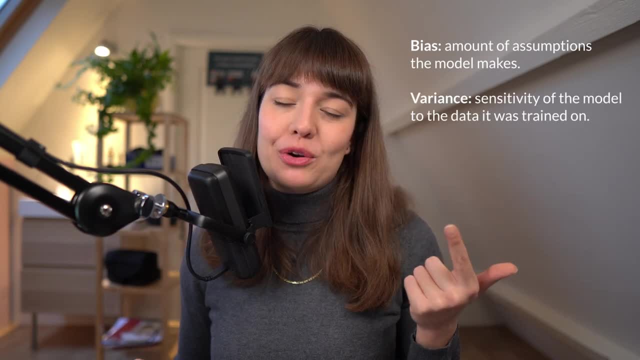 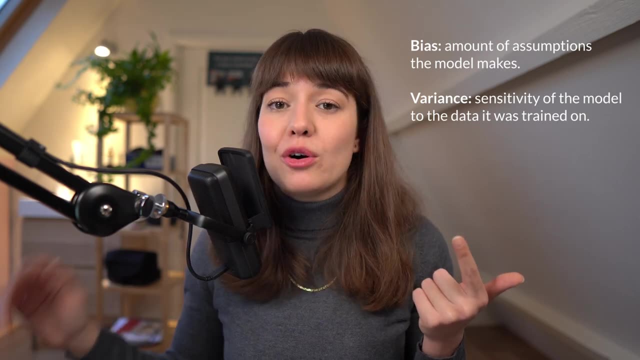 that will lead to underfitting Variance is the sensitivity of your model to the data that it is being trained on. If it has high sensitivity, that means you have high variance and that means that you're overfitting To deal with high bias. what you can do is to train your model more or increase. 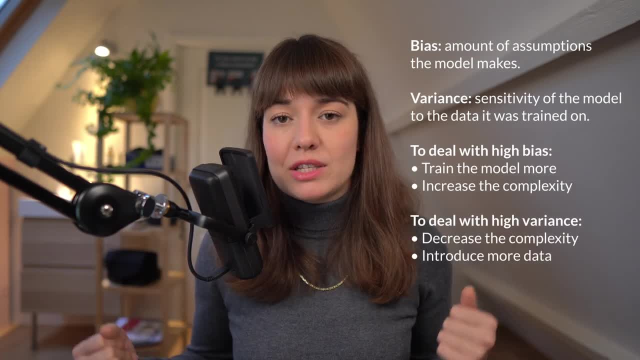 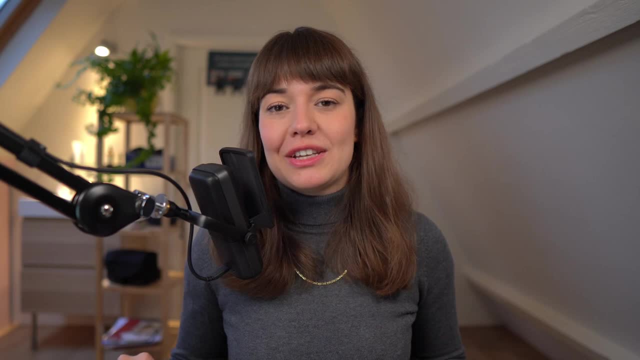 the complexity of your model, Whereas to deal with high variance, what you need to do is to decrease the complexity of your model or introduce more data to your training. If you understand all of this, that means you have a good understanding of bias and variance. 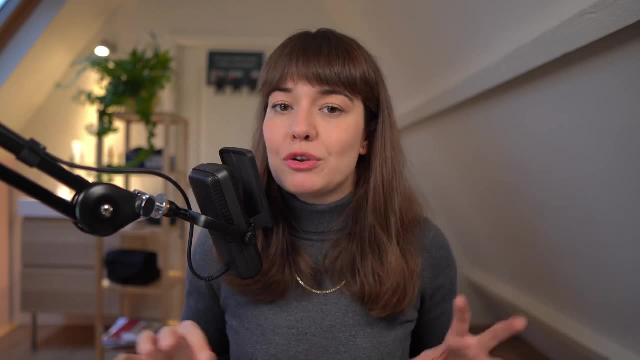 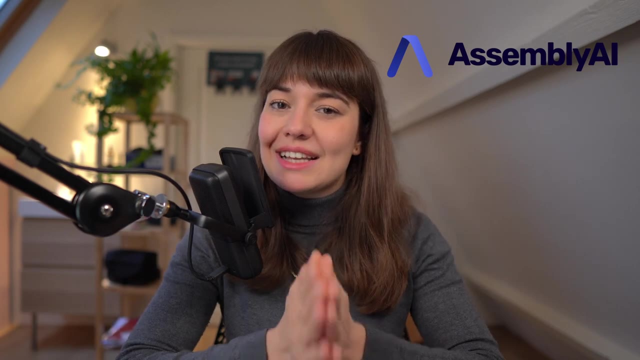 From now on, it will be easier for you to understand what to do when your model is underfitting or overfitting. Thanks for watching and I hope you enjoyed this video. If you liked it, don't forget to give us a like and maybe even subscribe. We would also love to hear about your 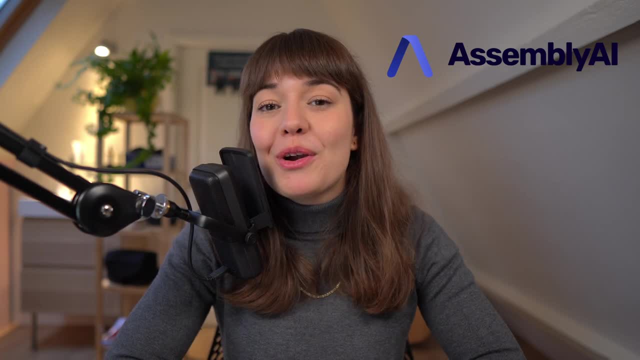 questions or comments in the comments section below. But before you go away, don't forget to go grab your free API token from Assembly AI using the link in the description. Have a nice day.